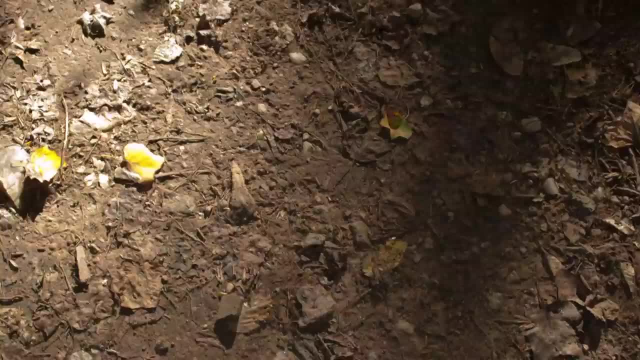 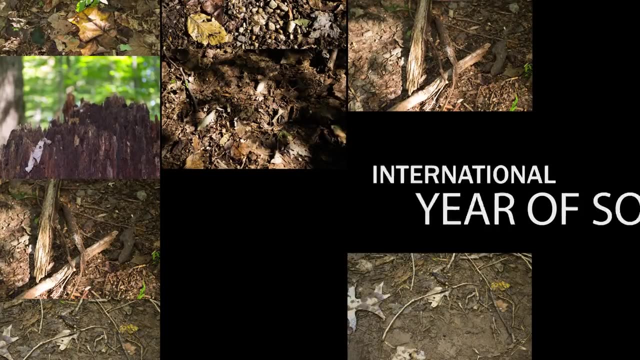 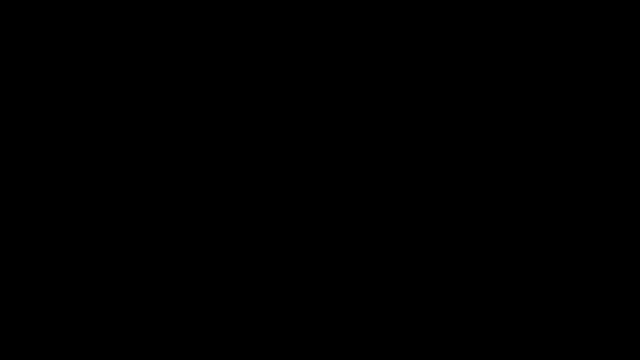 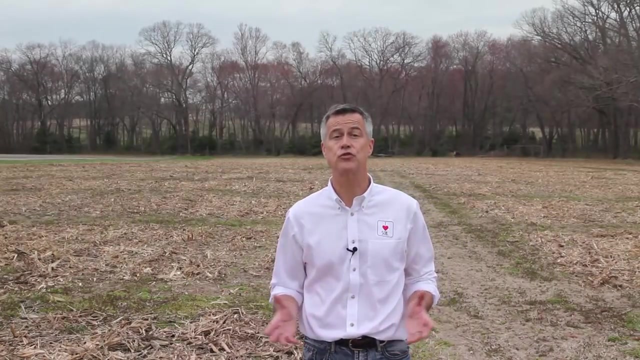 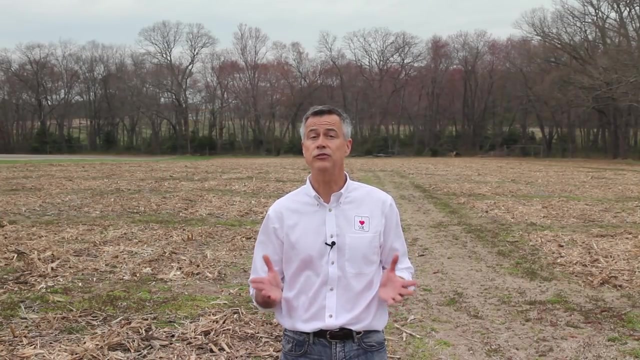 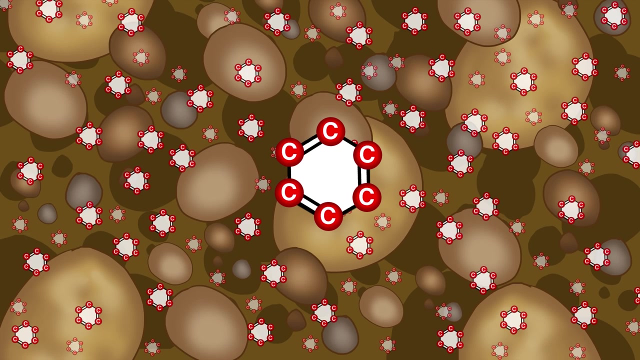 What does soil have to do with climate? Plenty Soils help moderate global temperatures, store carbon and can preserve records of past climates. Recent studies have shown that carbon is stored in healthy soils. Organic matter in soil holds large amounts of carbon, which is a major component of greenhouse. 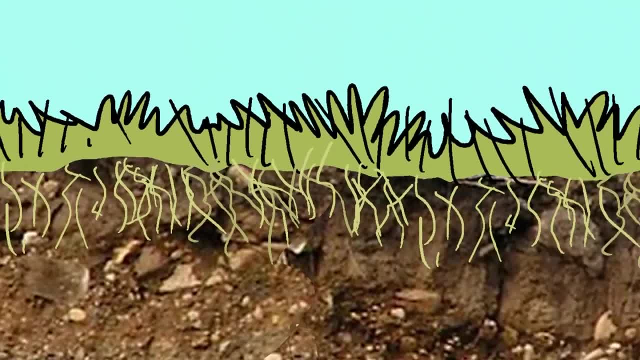 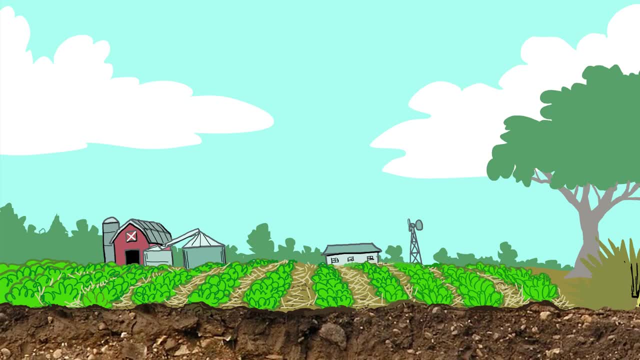 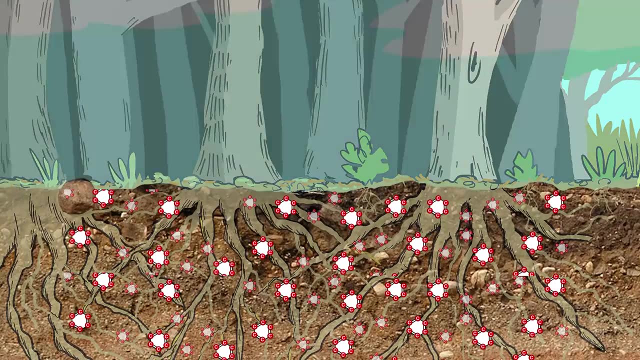 gases such as carbon dioxide and methane. Replanting forests, protecting and restoring wetlands and good agricultural practices can all help soil store more carbon, keeping it out of our atmosphere. Alternatively, deforestation, draining of wetlands and poor agricultural practices 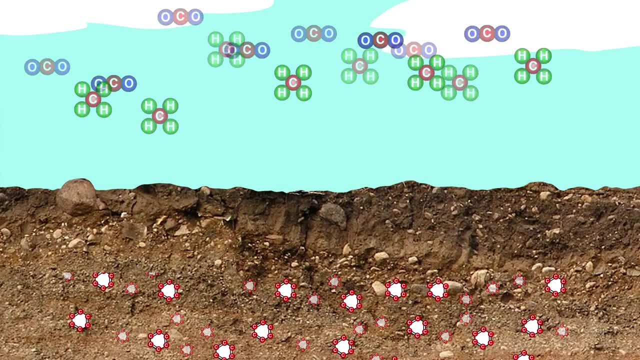 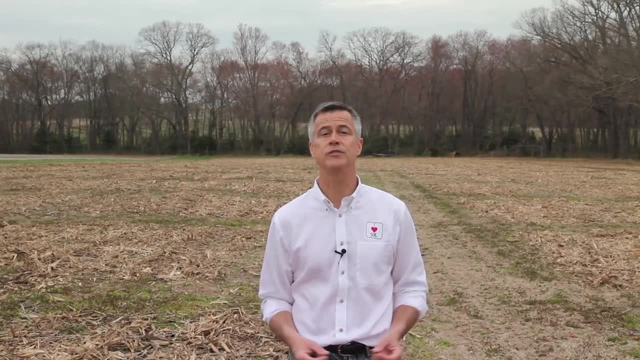 can release large amounts of carbon into the atmosphere, where it can contribute to climate change. One of the major influences in soil formation is the climate in which that soil was formed. Because of that, certain features found in soils preserve a record of climates in the. 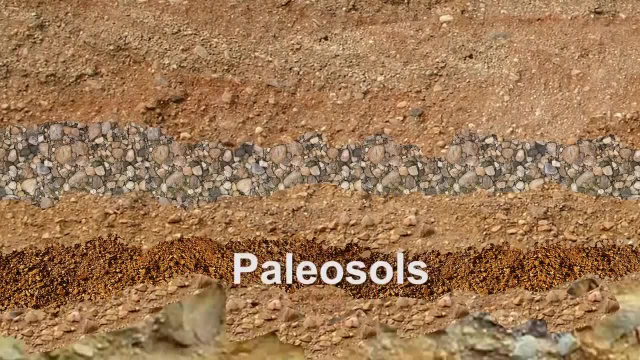 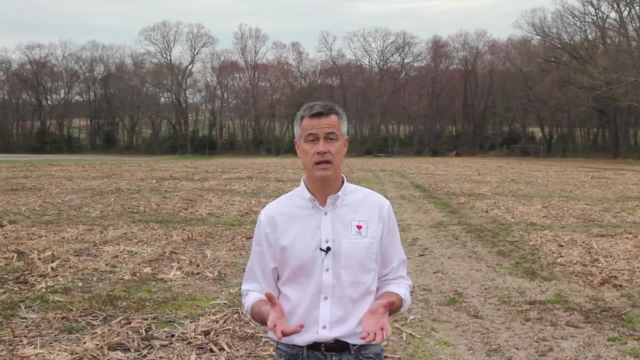 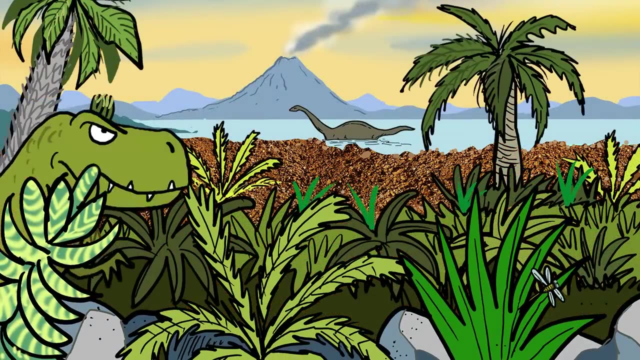 past. Old buried soils called paleosols are ideal climate records because in many cases they've been isolated from current soil forming processes and preserve features of the climate long ago. Paleosols provide a record of whether conditions were warmer or colder, or wetter or drier. 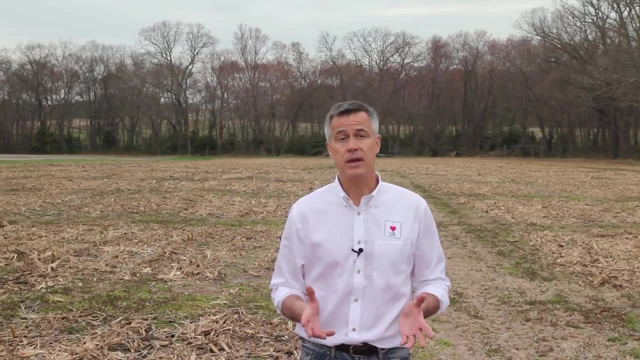 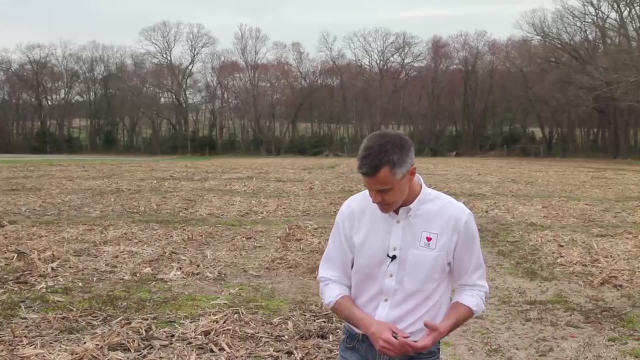 at the time they were formed. Knowing how to interpret the features found in paleosols provides scientists with a powerful tool to help reconstruct the climates of the past. Desertification is the rapid loss of topsoil and the loss of plant life on productive land. 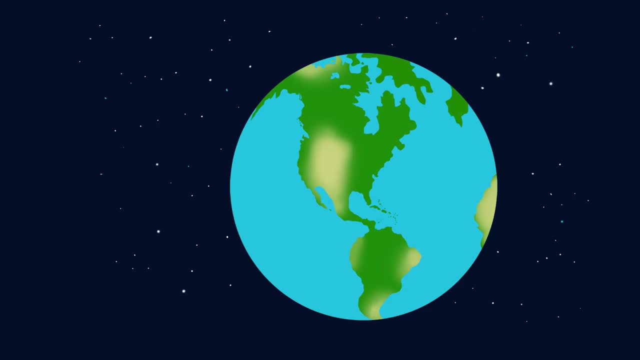 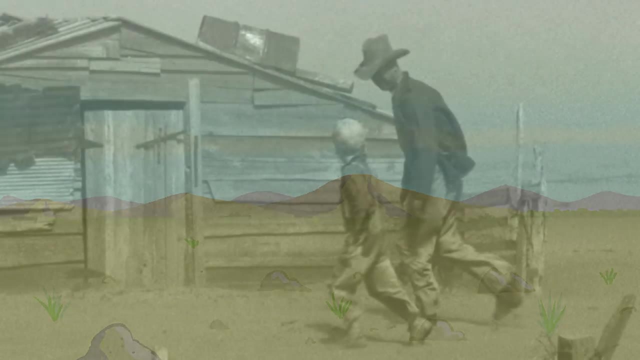 in arid and semi-arid regions of the world. One third of the Earth's land area in more than 100 countries, including here in the United States, is at risk of desertification. The historic Dust Bowl of the 1920s and 30s was a result of desertification caused by 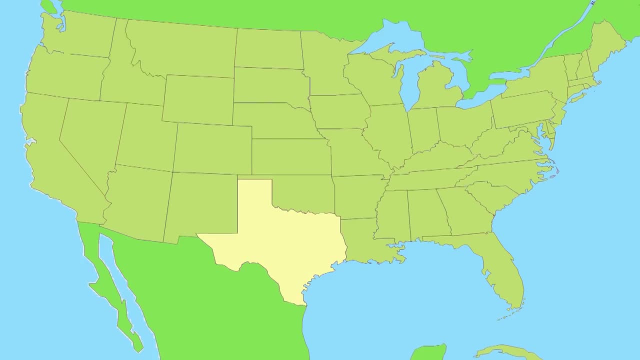 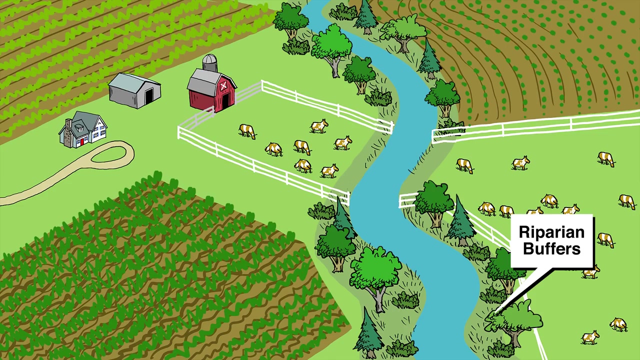 overgrazing and excessive tailage of soils. in Texas, Oklahoma, Kansas and Colorado, Most desertification can be prevented by following good farming and property management practices. We need to prevent desertification so we can continue to have fertile soil to grow food.